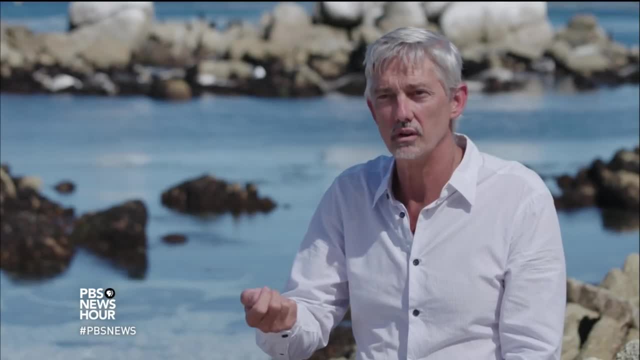 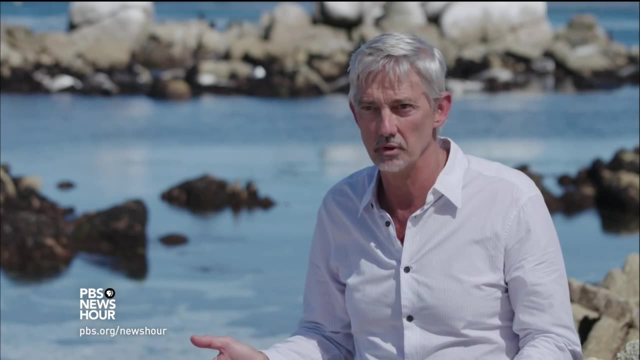 It's not a problem, you can just turn around very quickly. It's a problem that once it gets really bad enough so that it is having an incredible global effect, there's nothing you can do about it. You have to stop it before that point. 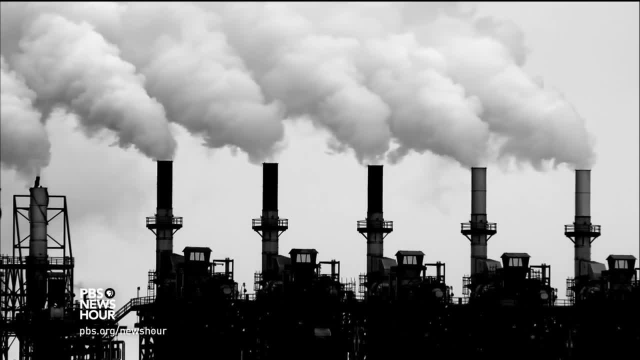 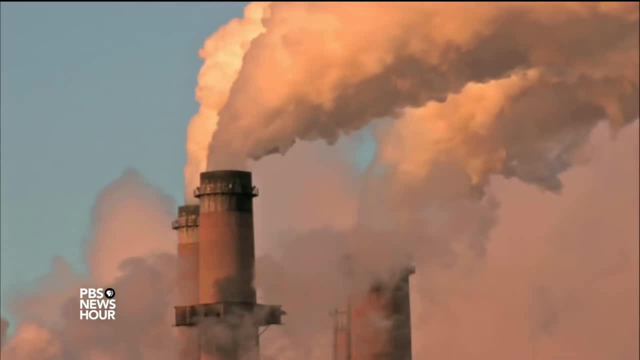 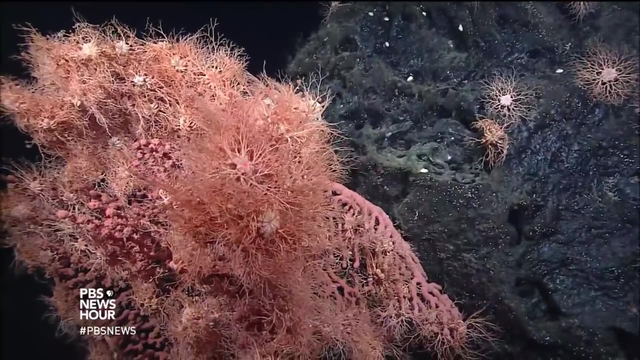 The increase in acidity is largely the result of people burning coal, oil and other fossil fuels. That pumps massive amounts of carbon dioxide into the atmosphere, which then sinks into the ocean waters at a rate of 9 billion tons per year. The carbon dioxide robs the oceans of an essential element that corals and other animals need to thrive. 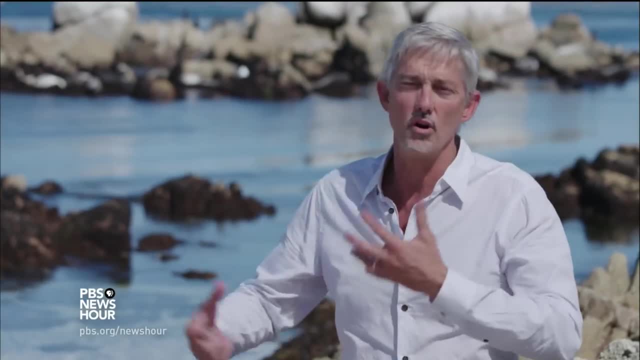 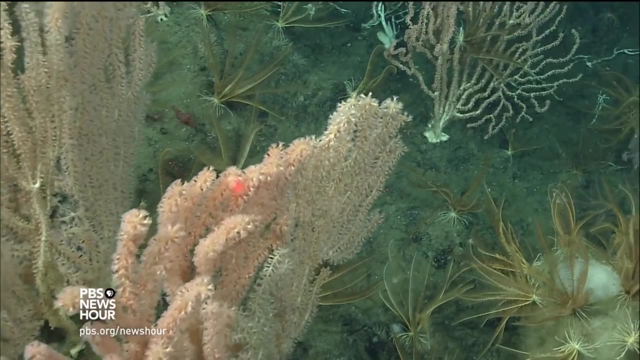 Corals make skeletons. That's the white part of a coral reef And the skeletons are made of calcium carbonate. Calcium carbonate tends to dissolve if the acid level in water gets too high. Calcium carbonate tends to dissolve if the acid level in water gets too high. 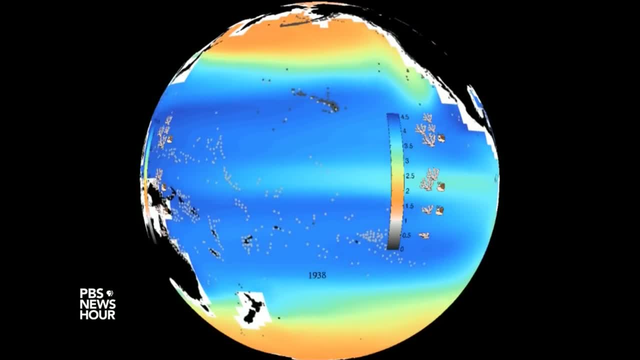 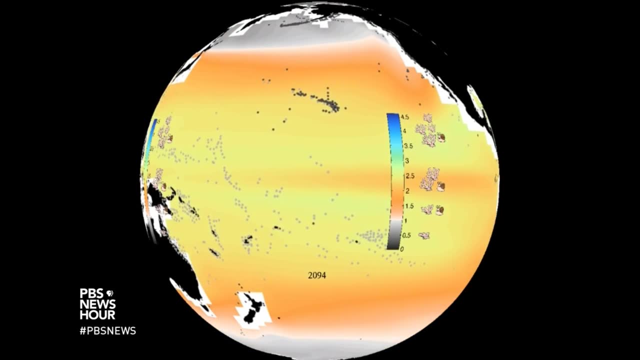 Calcium carbonate tends to dissolve if the acid level in water gets too high. This model shows how the ocean chemistry has changed since 1885 and how it is expected to change over the next 80 years. The blue represents ocean conditions good for shell and coral growth. 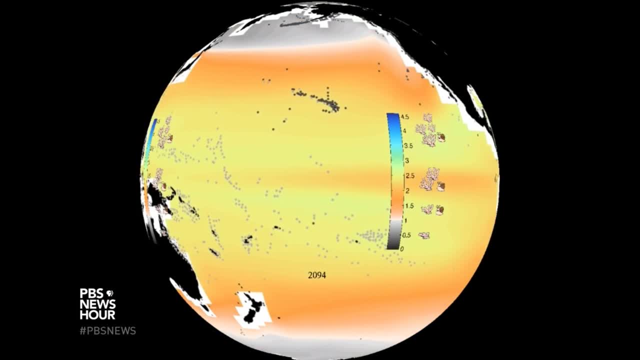 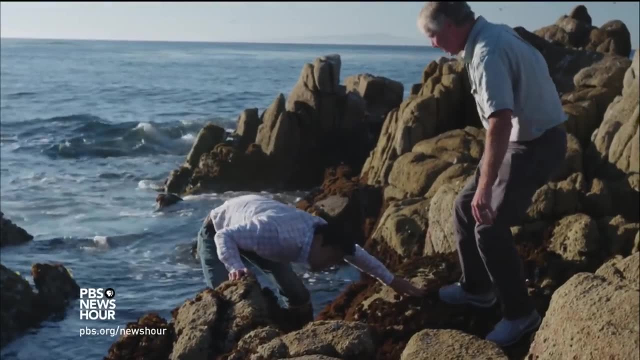 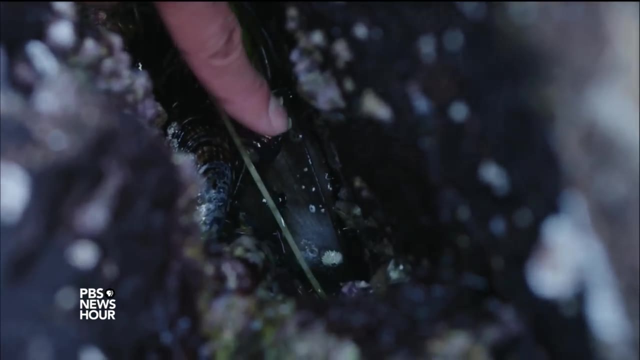 The orange represents conditions that make it difficult for many animals to grow shells or skeletons. There's a few of them right here. Most of them might be deeper. Jim Barry is a senior scientist at the Monterey Bay Aquarium Research Institute. He's looking at the effects of ocean acidification on a variety of sea life, including deep sea coral. 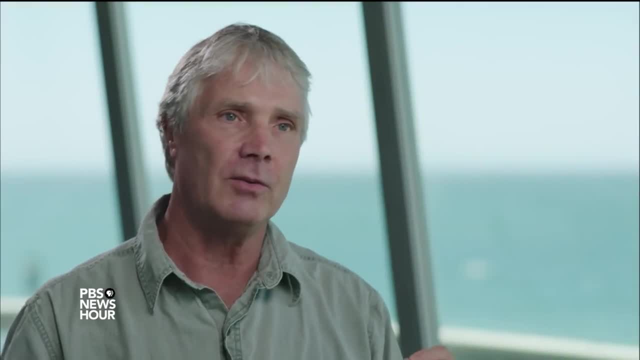 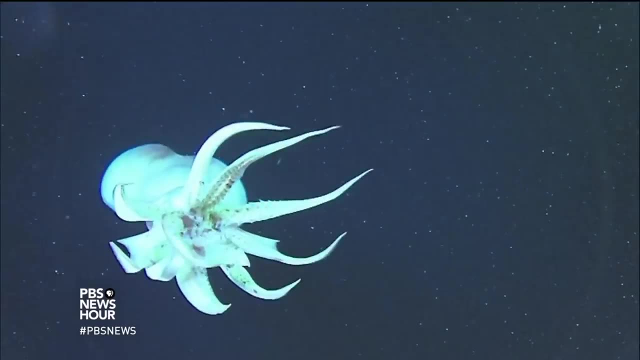 The ocean critters out here are faced with a faster and larger change in ocean chemistry than they've seen for 30 to maybe 300 million years through much of their evolutionary history. Barry says if one species suffers, an entire food web can suffer. 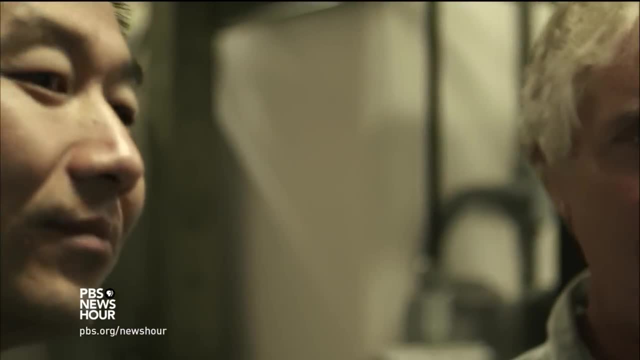 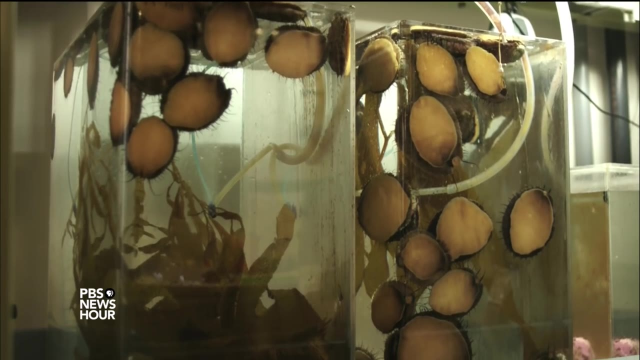 We can just measure this motility rate. Barry and researcher Charles Bock are studying how ocean acidification affects sea life. They're studying how ocean acidification affects abalone, specifically whether it interferes with the ability of the shellfish to reproduce. 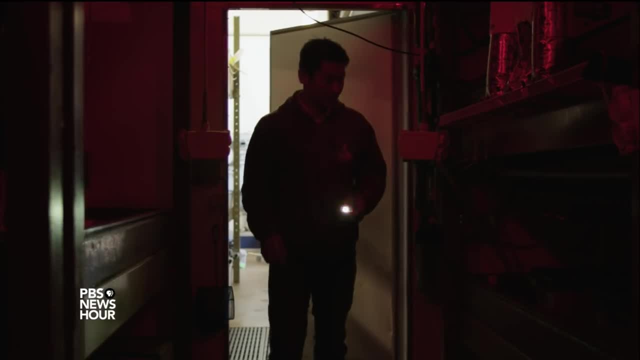 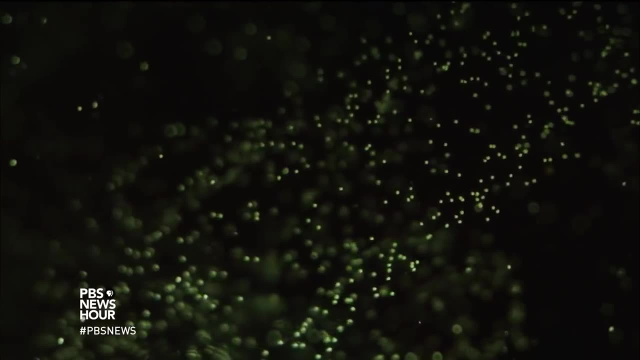 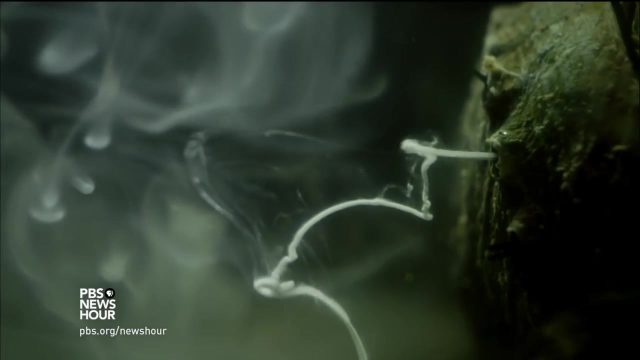 Inside a chilly lab, Bock is inducing female abalones to spawn. Each female releases streams of small green eggs through its respiratory holes. An abalone can spawn tens of thousands of eggs at a time. In one tank are the females, In another the males? 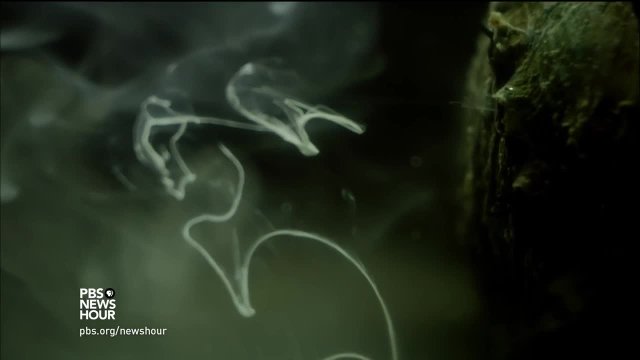 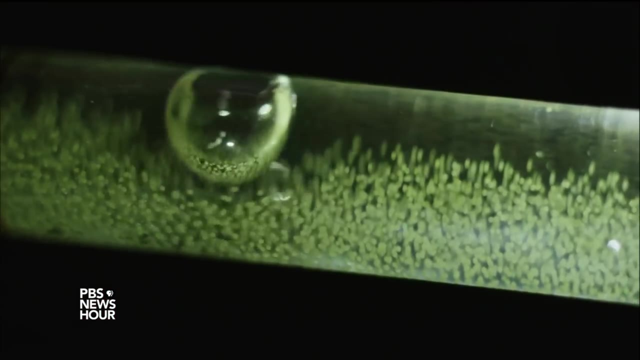 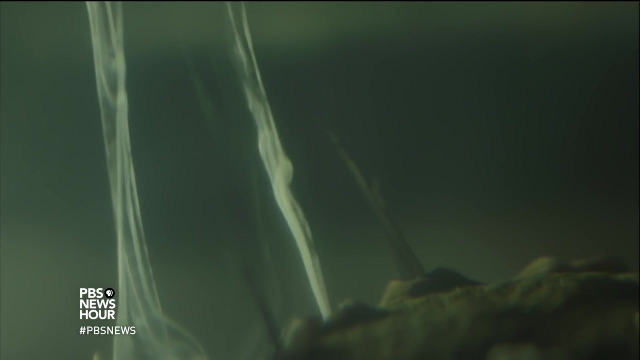 What you're seeing is puffs of cloud. These are the white streams that are the sperm being released. Bock and Barry are putting the eggs and sperm together in water with varying levels of acidity to examine how it affects fertilization. Maybe what we saw in the last experiment, where fertilization was lower in low pH. maybe it's because the sperm aren't swimming as fast. 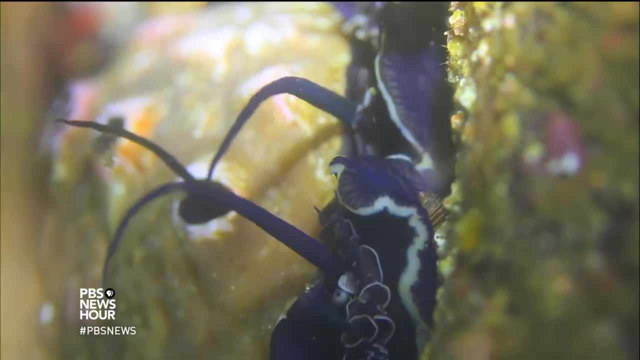 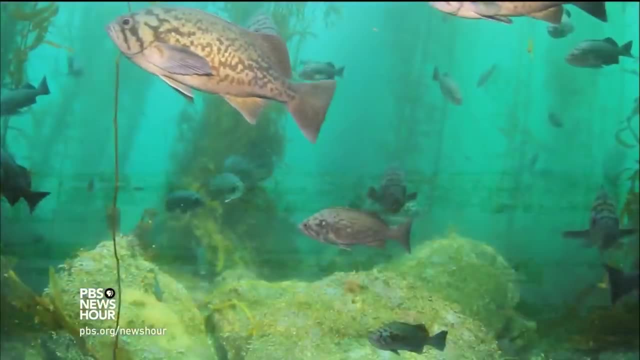 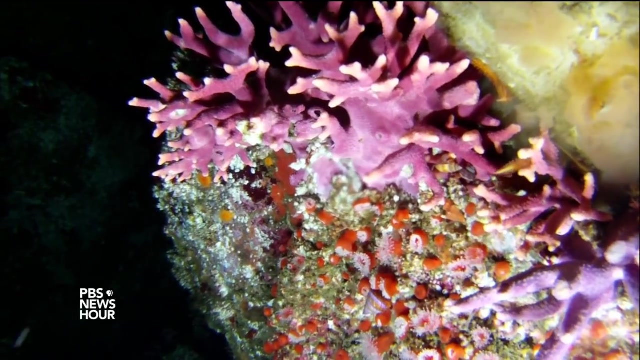 Their research suggests that ocean acidification significantly reduces the abalone's fertilization rate. Abalone are an important source of food for sea otters and in turn help keep kelp forests in balance. We know that ocean acidification is huge. This is one of the biggest things that happened to this earth in the last many tens of millions of years. It's a huge environmental change that's happening right in front of us. Terry Sawyer runs Hog Island, an oyster farm on Tomales Bay 30 miles north of San Francisco, And this is a big Pacific oyster. This is how big they will get. 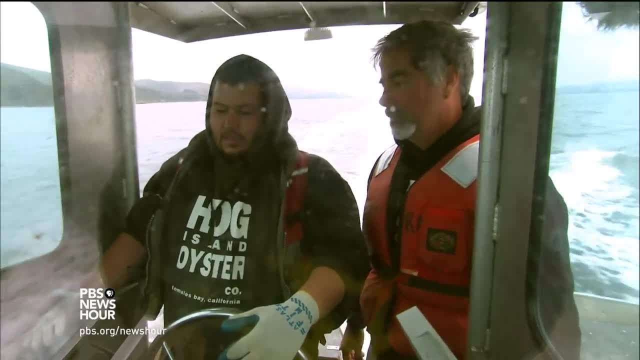 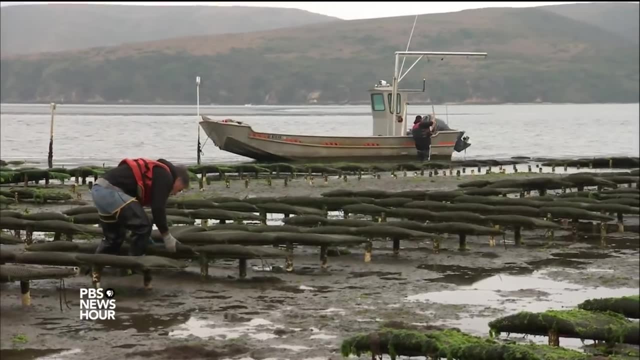 Sawyer says ocean acidification is already affecting his business. It's really scary. It's a very scary place to be. The wake-up call for him came in 2005.. That's when there were massive die-offs at oyster hatcheries along the Oregon and Washington coasts. Those hatcheries supplied Sawyer and many other shellfish farmers with the seeds and larvae they needed to grow their oysters. The larvae was completely dying and their seed was completely dying. It's not a way to run a business. Sawyer says he's concerned not only for his business but for all the animals who live in or depend on the oceans. 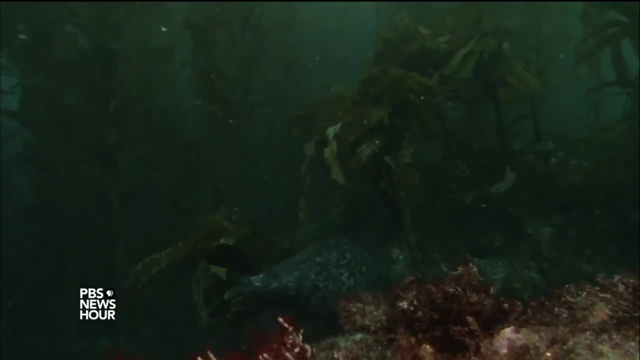 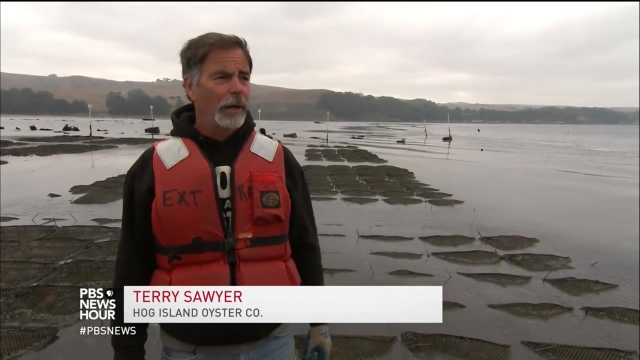 It feels like we're in the position being the canary in the coal mine. The thing is, I'm holding the canary And so I've got a responsibility to say: well, all right, we have symptoms here that you know. that animal just died. 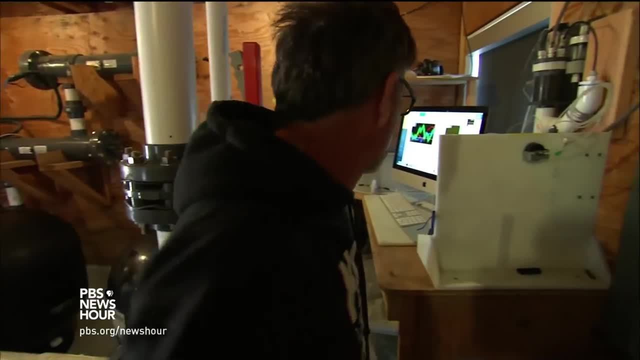 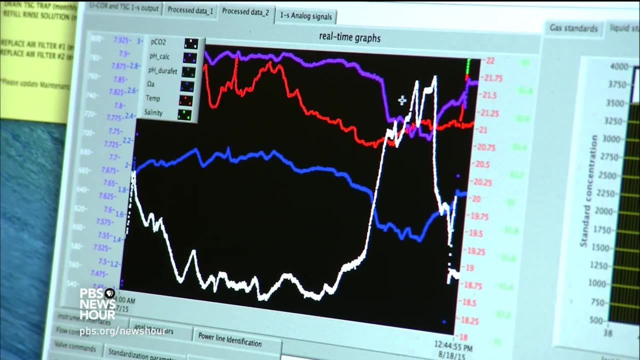 Okay, what are we going to do now? Sawyer and researchers from the University of California Davis are now monitoring the water quality in real time. Purple line is P8. The data helps Sawyer and other oyster farmers in the area adjust planting schedules. 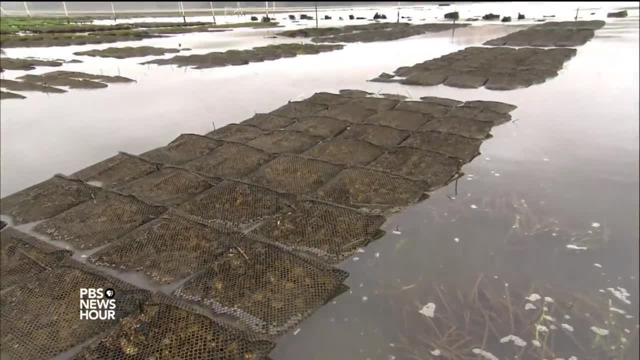 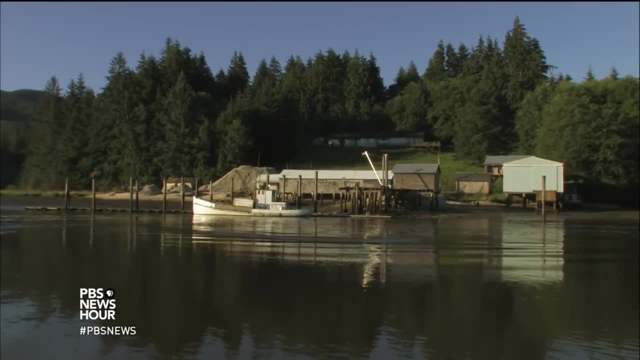 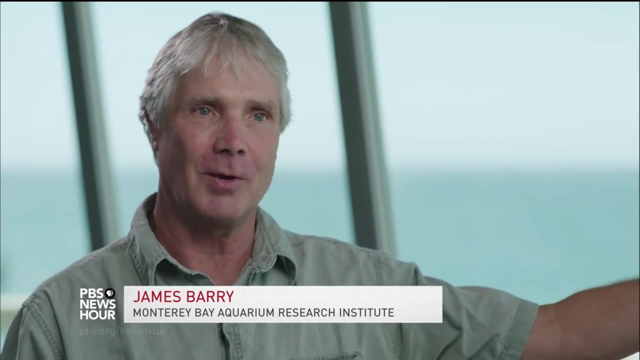 To prepare for changing conditions, Hog Island is building its own hatchery. A large oyster hatchery has already moved to Hawaii, leaving the more caustic waters of the Pacific Northwest. That's great for that hatchery, but what does it mean for all the animals that are already living there? 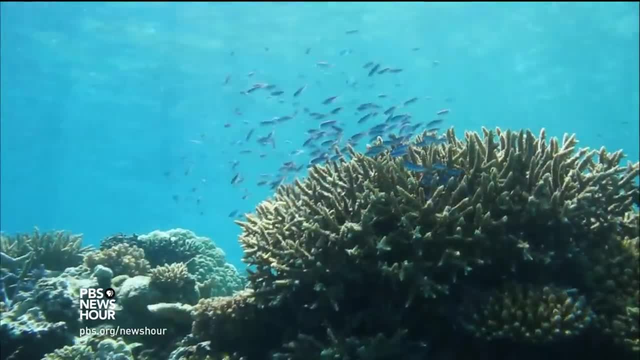 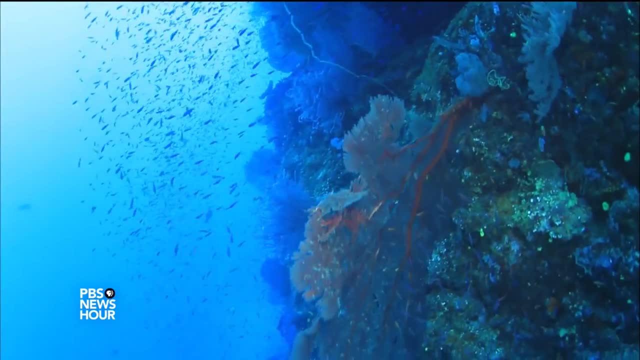 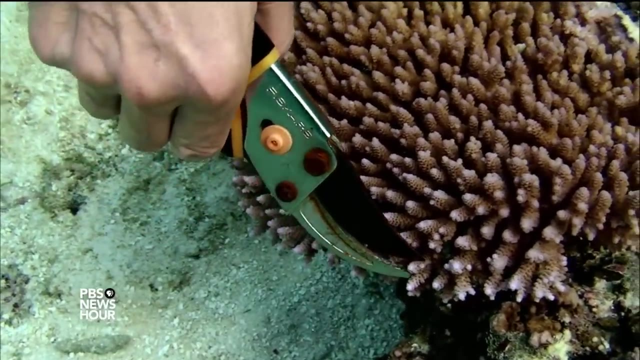 They can't move. Jim Barry fears it may already be too late to save coral reefs. He points out that four of the last five big extinctions on Earth included ocean acidification. Scientists say it is unclear if ocean acidification has reached a tipping point.